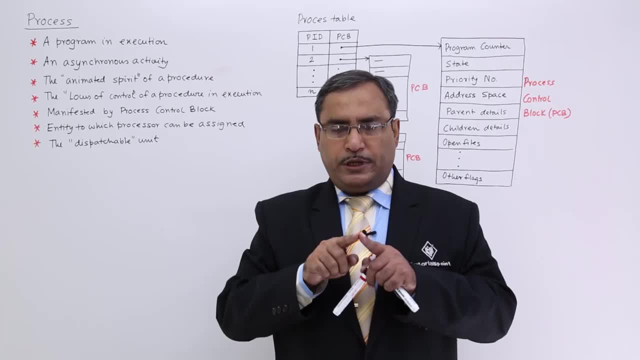 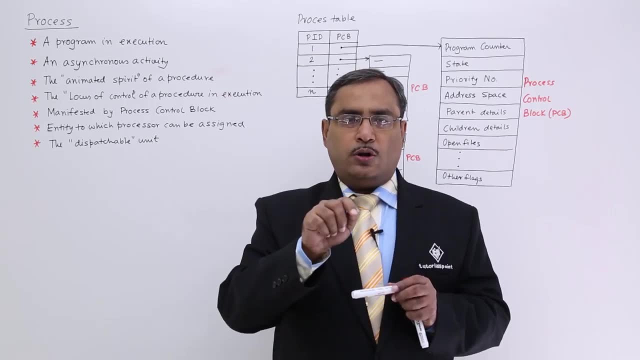 control flow. There will be some conditional boxes will be there where the control will be directed either towards the ìyesî column, ìyesî edge, or it will be coming to the ìnoî edge. So obviously there will be different sequencing will be there in a process. 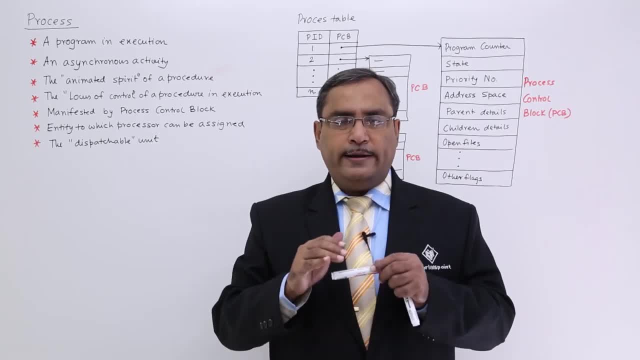 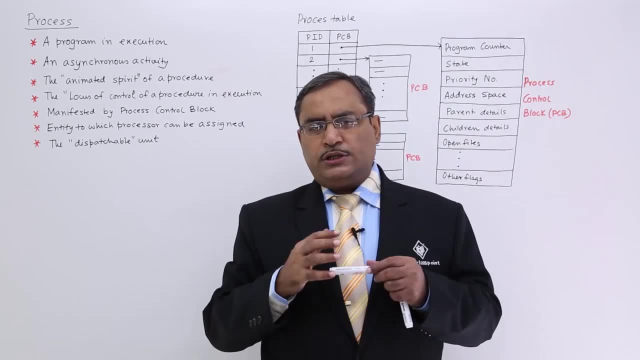 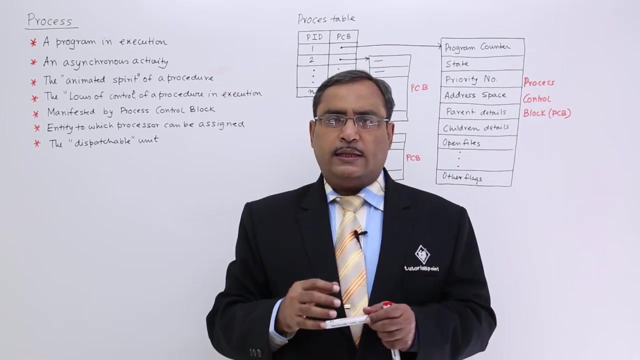 but the process will have some locus of control and it is not a deadly thing, but it is having a spirit Manifested by a process control block. Process control block will keep the process related information. Actually, process control block is nothing but one data structure which will keep multiple different information regarding a particular 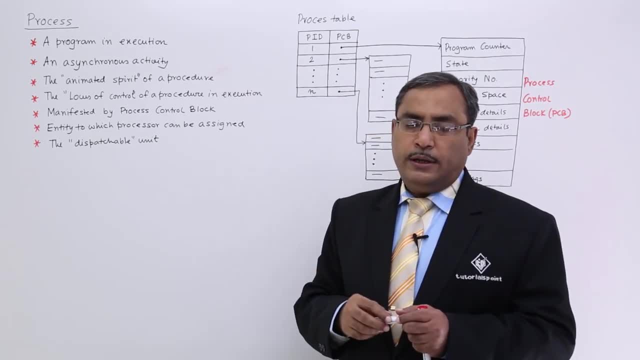 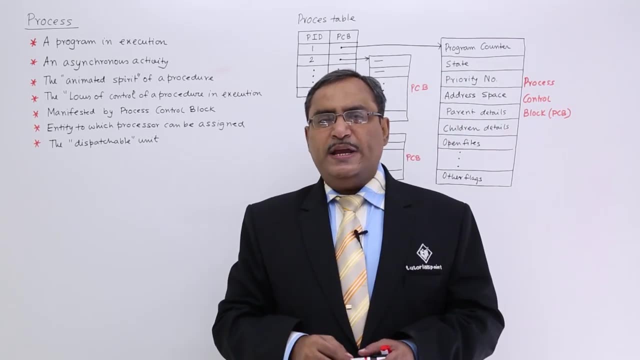 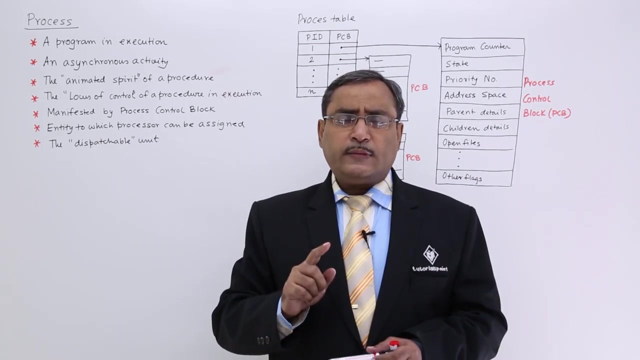 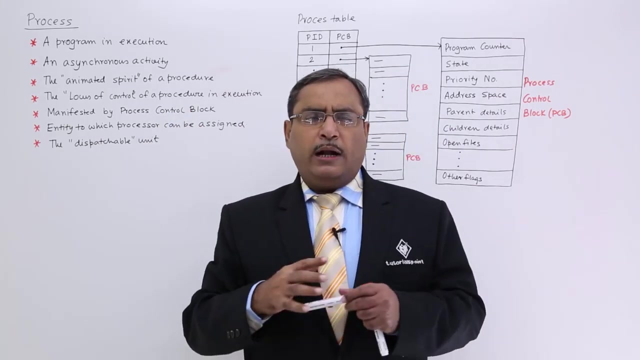 process. so whenever a process will get executed, then each and every process will have one unique identification number and that is known as the pid process identification number, and against each and every process, there will be one pcb, that is a, that is a process control block pcb, and that will contain multiple different information regarding the process i am having. 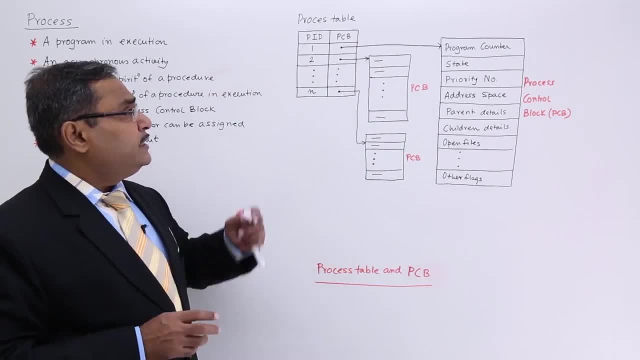 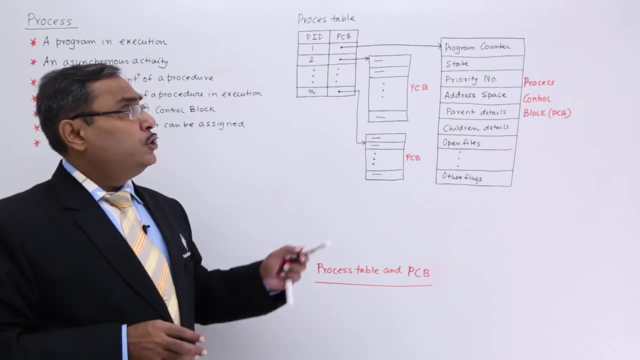 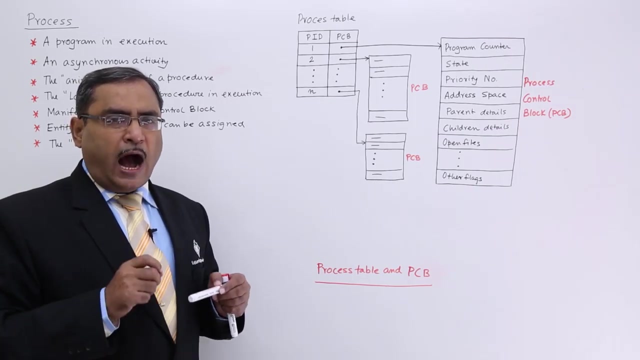 a separate diagram on this particular pcb. you see, this is known as a process table. so here we are having n number of processes have got loaded onto the computer's memory. so this process table is fundamentally is having two columns. one is a pid which will hold the unique. 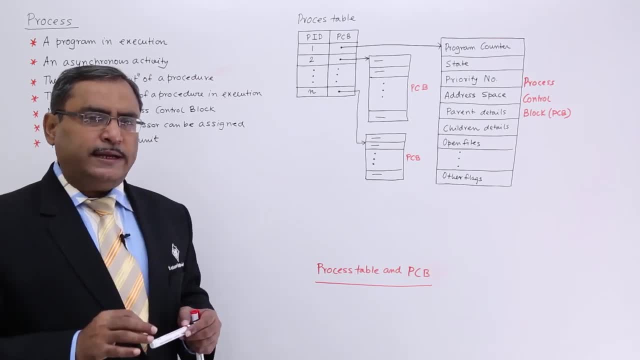 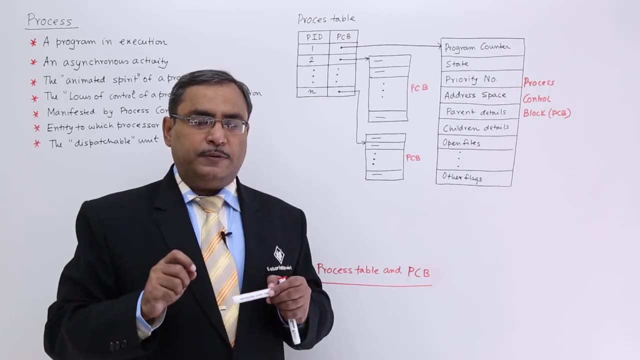 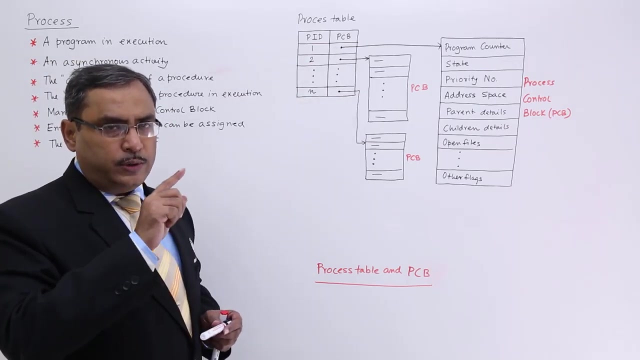 identification number of the process. the number will be assigned to the process arbitrarily by the computer and the process table will be assigned to the process by the computer. but it is quite confirm that the number will be unique at that instant of time and another column will be there where it will be having a pcb pointer, where it will be pointing to. 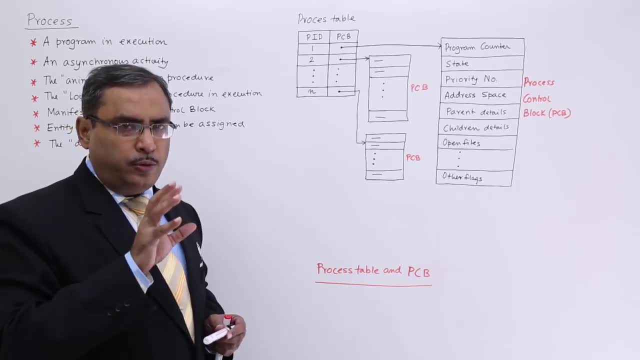 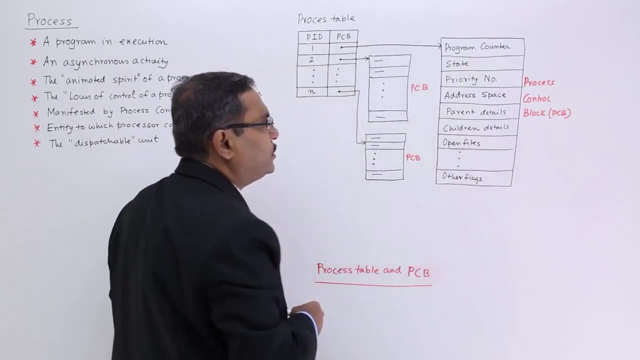 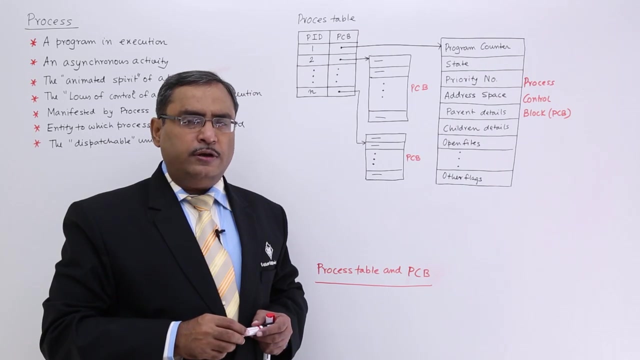 a certain memory block where the process related information will be kept in a data structure known as a process control block, pcb, so it can contain some set of information like program counter. you know that program counter is nothing but a register which will point to that particular memory location from. 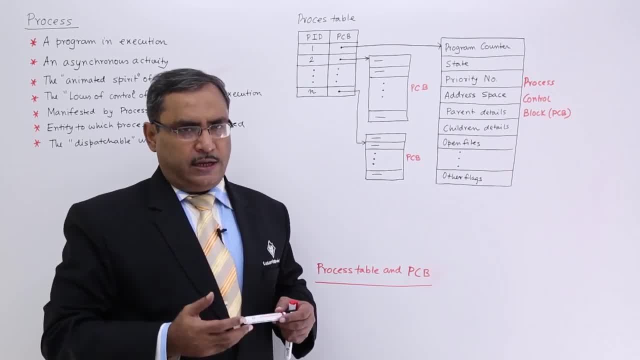 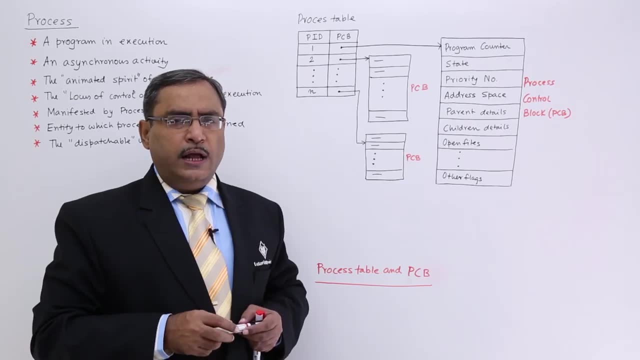 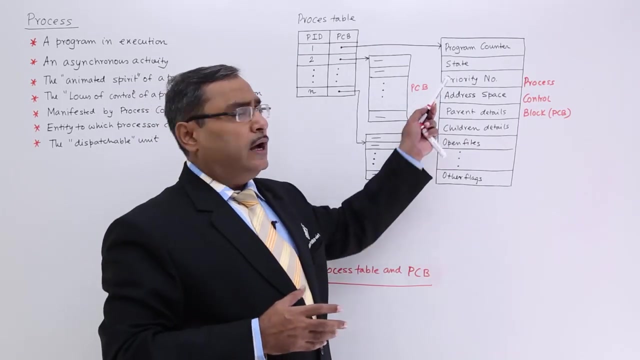 where the next instruction or data is to be placed, so program counter will be there. the current content of the program counter state of a process in the next videos will be coming for the different types of state possible for a particular process. so this particular state can be a block state, can be a running state and so. 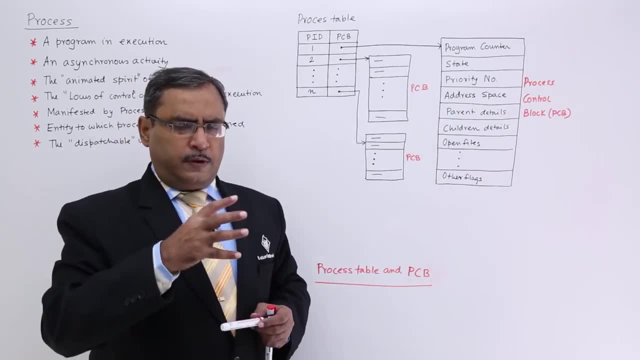 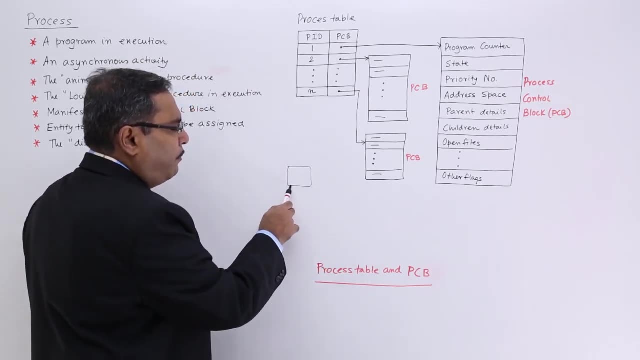 on priority number whenever multiple multiple resources are there- and let us trying- is one resource when having the multiple resource. i am consideration on this one. multiple priority processes are competing for this particular resource. Say, P1 is demanding this particular resource R1 and P2 is demanding this particular resource- R2 at the same time. And this resource. 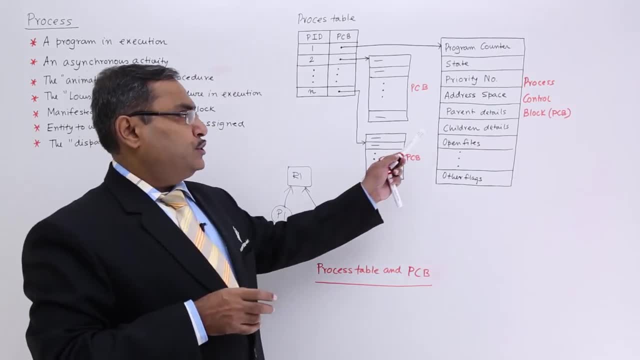 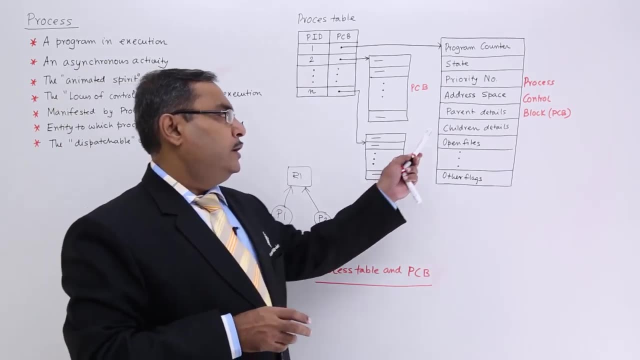 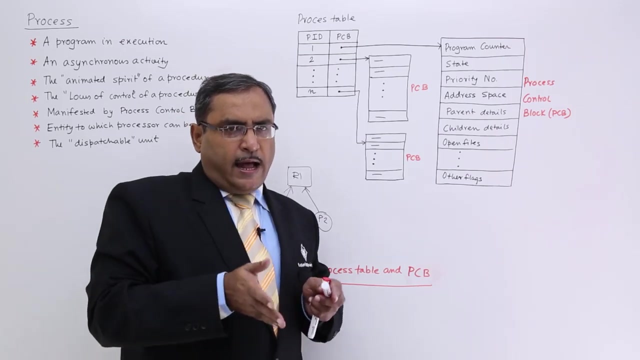 is non-shareable. In that case, the process priority number will decide that which process will get an access over this particular resource R1.. A process will get created from another process, So this process, the current process, will have the PID and its parent process will. 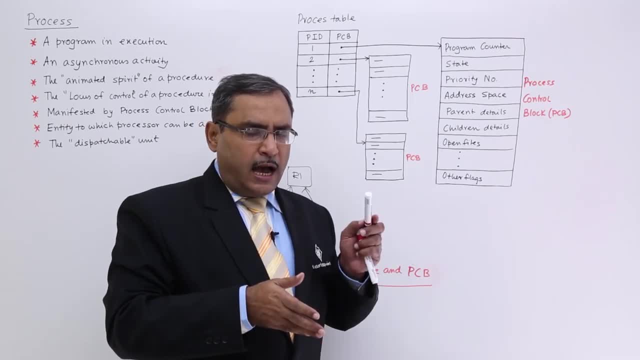 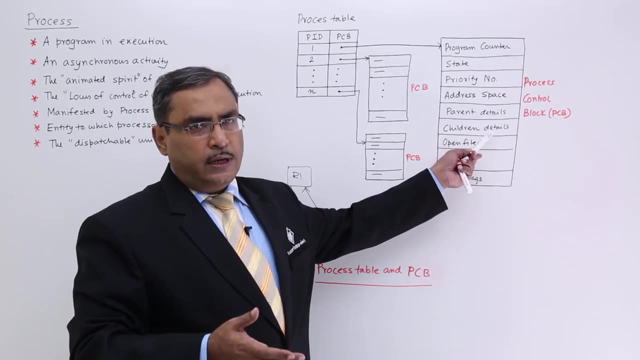 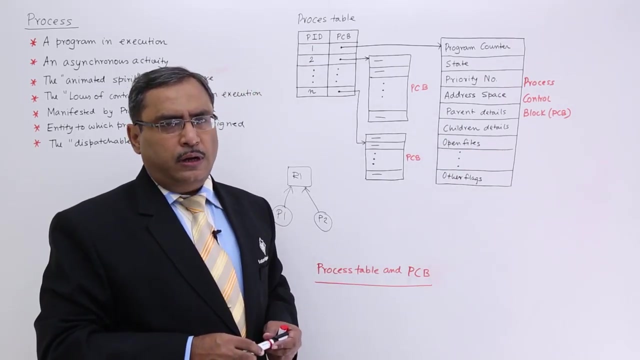 have the PPID, that is a parent process identification number, And a process can create other child. So in that case the children details will be there. So all the children, their corresponding details, will be kept in the PCB. How many files are opened for that particular process? 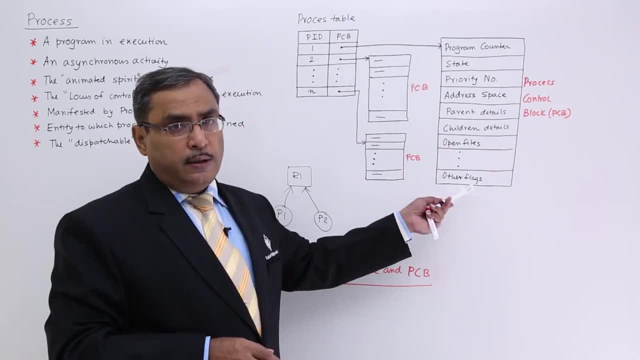 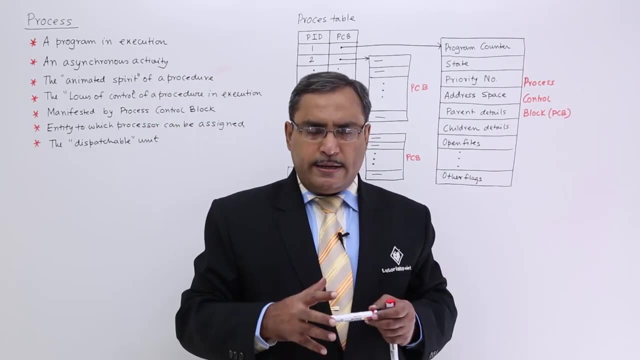 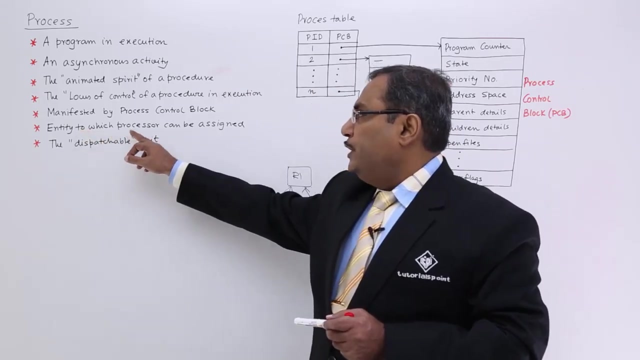 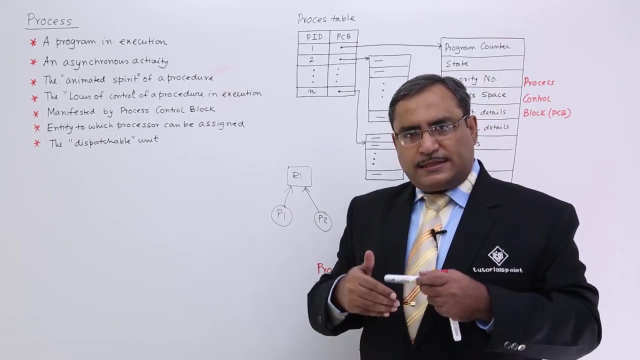 execution, The trace will be kept in this particular PCB and other flags. So these are the different set of information that will be maintained by the data structure PCB against each and every process Entity to which a processor can be assigned. It is a very interesting this particular line, that is, processor can be assigned to a process. 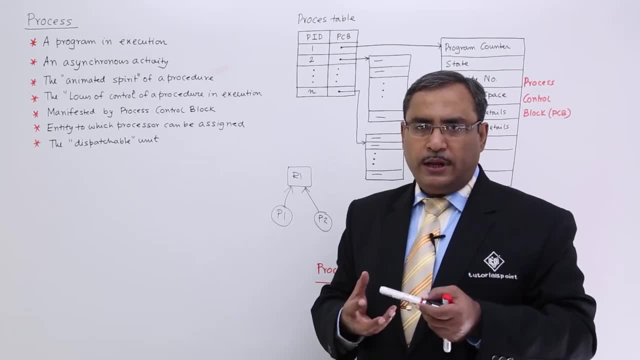 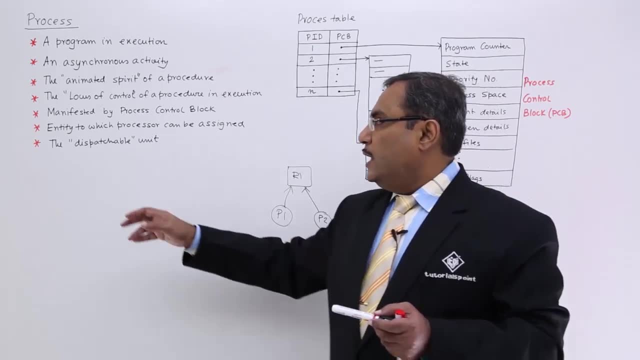 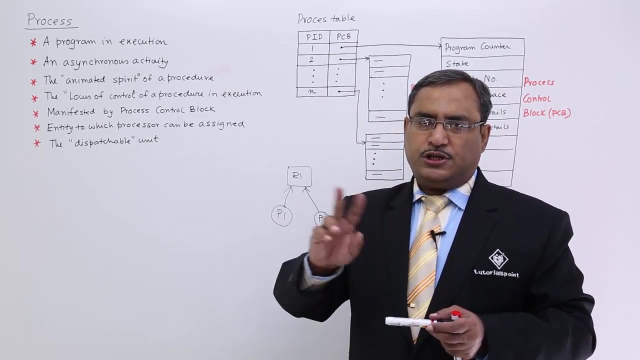 for execution. Processor means the CPU, means the hardware, and process means a software. So processor will be assigned to a process to get the process executed And it is a dispatchable unit. Assigning the CPU to a particular process, this particular action is known as dispatch. So process is a dispatchable unit. That means the CPU can. 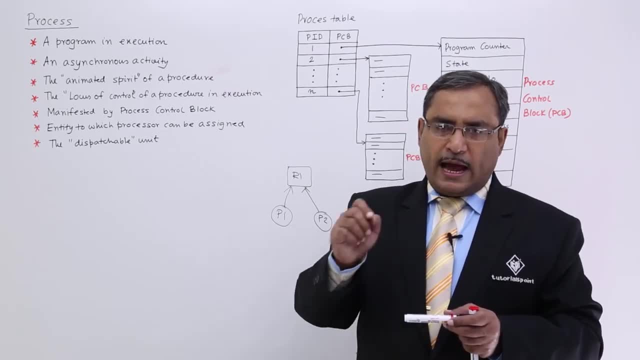 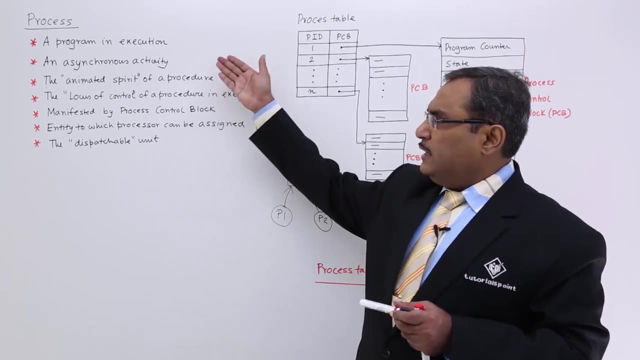 be assigned to a process. So this particular action or activity is known as dispatch. So that is why process can be defined as a dispatchable unit. So you see, in the various different ways we can define a process and all the details. 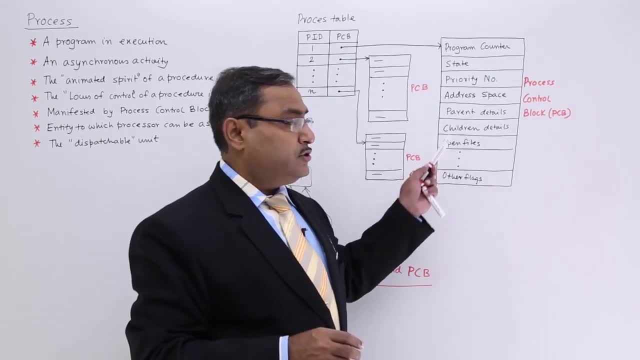 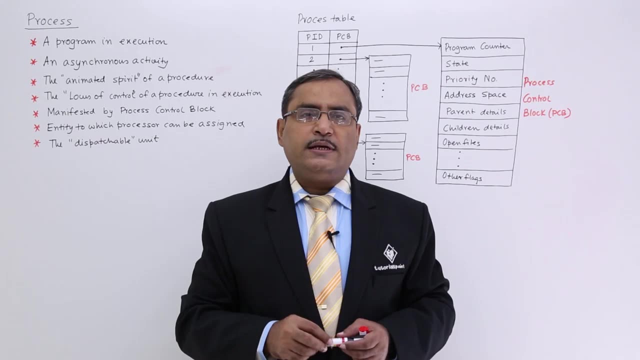 of a process will be kept kept in the PCB and it is a data structure. some of the fields we have mentioned here. Please watch the next video on this particular process. we will be discussing other features of process. Thanks for watching this video.